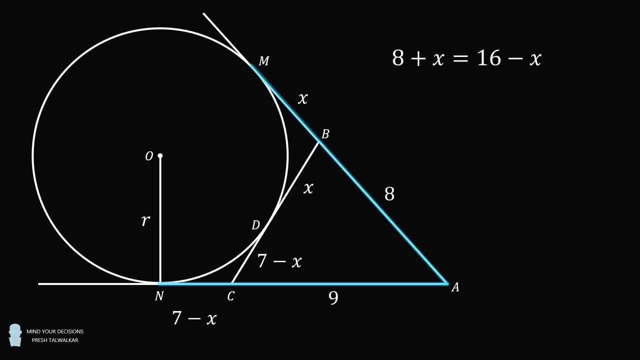 so we have: 8 plus x is equal to 16 minus x. This means 2x is equal to 8, so that x is equal to 4.. Substitute in x is equal to 4.. This means BD and BM are equal to 4.. 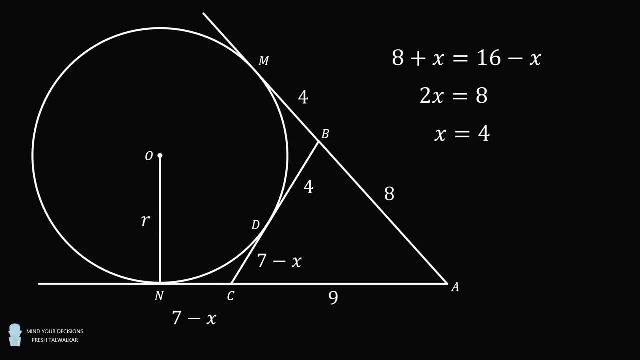 Then DC and CN are equal to 7 minus x, which means each of them is equal to 3.. Next, construct some line segments. Construct the radii OM and OD. Each of these has length equal to r. Each of these radii is also perpendicular to the line that's tangent to them. 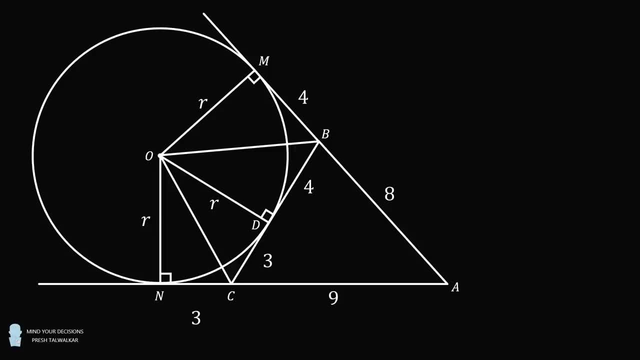 Then construct OC, OB and finally OA. We will now look at the area of some shapes. Let's get rid of the circle. Now consider the entire quadrilateral ANOM: Its area will be equal to an O plus AMO or ANO. 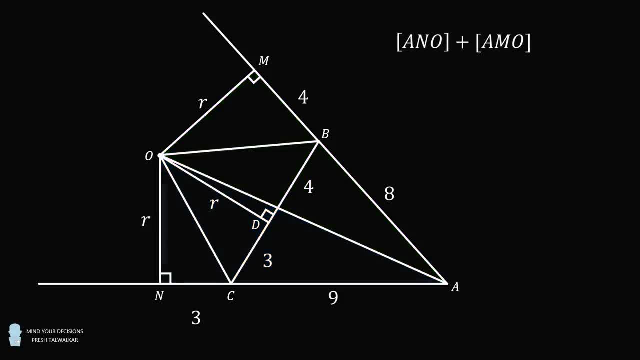 But we can also calculate the area in another way. The area of this quadrilateral will also be equal to the area of triangle ABC plus the area of triangle CNC. We can calculate this quadrilateral in another way. The area of this quadrilateral will also be equal to the area of triangle ABC plus the area of triangle CNO. 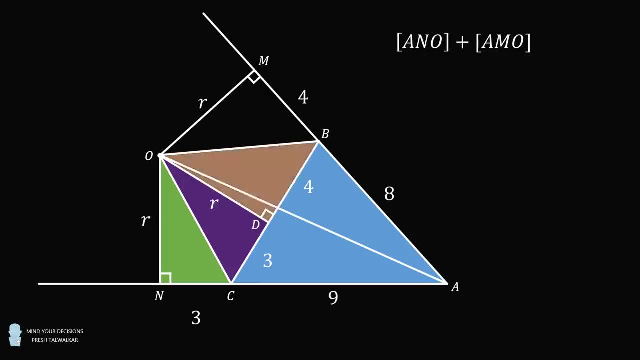 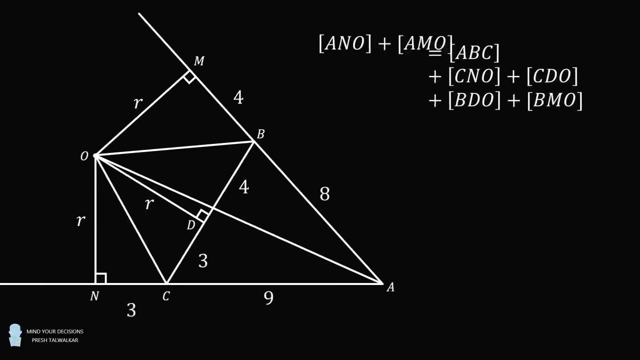 plus the area of triangle CDO, plus the area of triangle BDO, plus the area of triangle BMO. So we add up all these areas. So we have two different ways of expressing the same area. therefore, they're equal to each other. Let's now 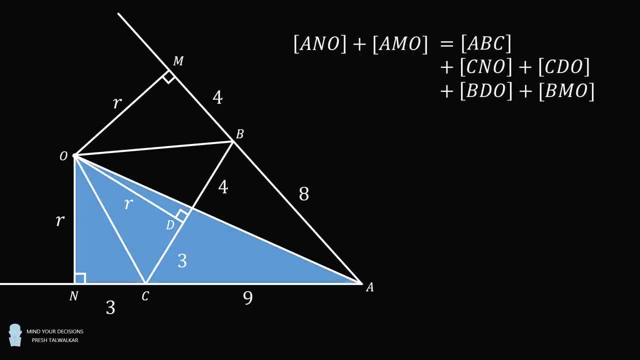 calculate each of these areas. The area of triangle ANO is equal to 12r over 2.. That will be the same area for the triangle AMO. We add these areas together and we get an area that's equal to 12r. Now let's calculate the areas of. 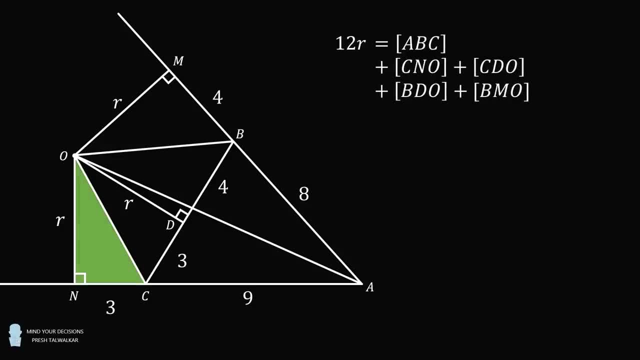 some of these other triangles. The area of triangle CNO is equal to 3r over 2.. That's the same for the area of triangle CDO. We add these two areas together to get a total of 3r. Then the area of triangle BDO is the same of the area of triangle BMO and 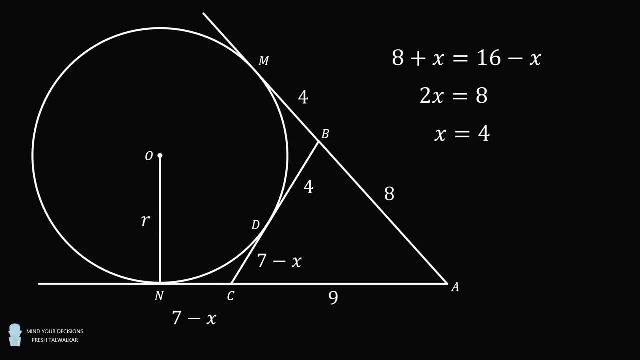 Then DC and CN are equal to 7 minus x, which means each of them is equal to 3.. Next, construct some line segments. Construct the radii OM and OD. Each of these has length equal to r. Each of these radii is also perpendicular to the line that's tangent to them. 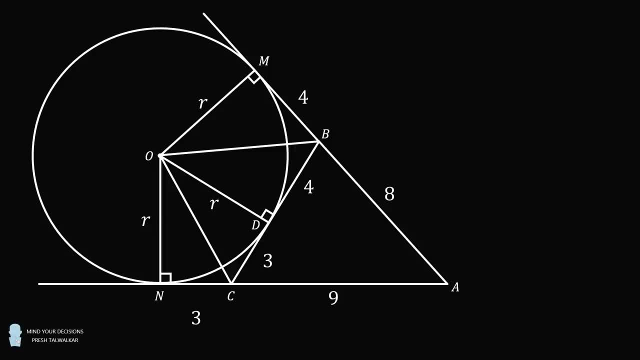 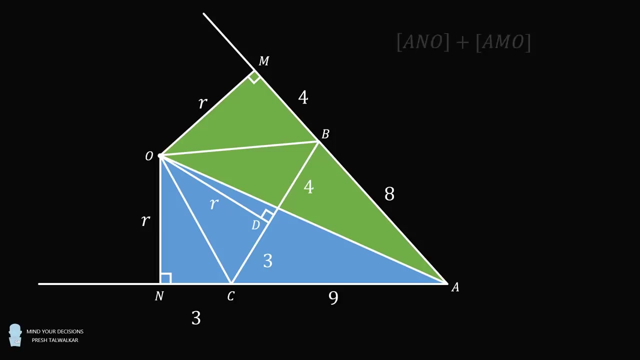 Then construct OC, OB and finally OA. We will now take a look at the area of some shapes. Let's get rid of the circle. Now consider the entire quadrilateral ANOM. Its area will be equal to the area of two right triangles. it'll be ANO plus AMO. 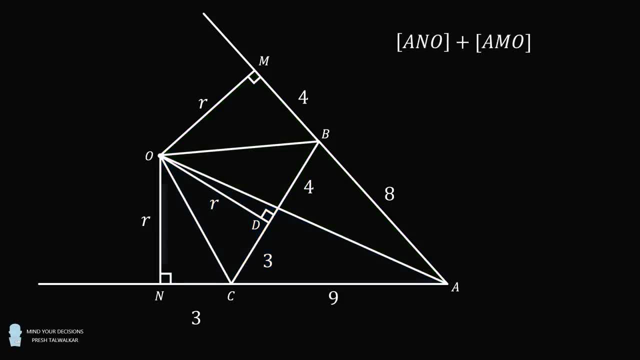 But we can also calculate the area in another way. The area of this quadrilateral will also be equal to the area of triangle ABC, plus the area of triangle CNO, plus the area of triangle CDO, plus the area of triangle BDO, plus the area of. 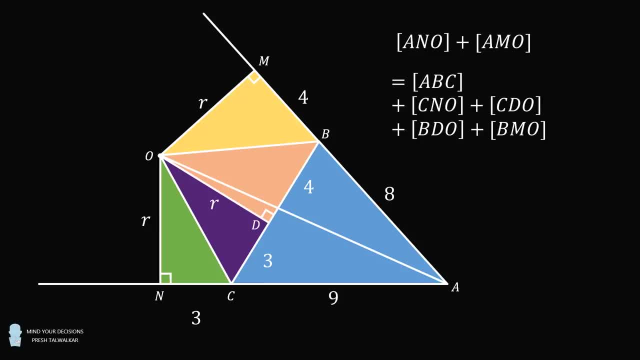 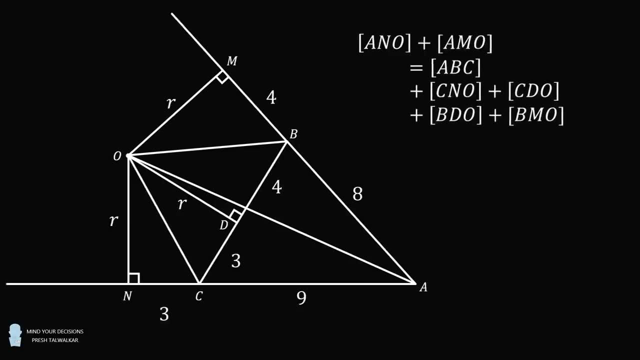 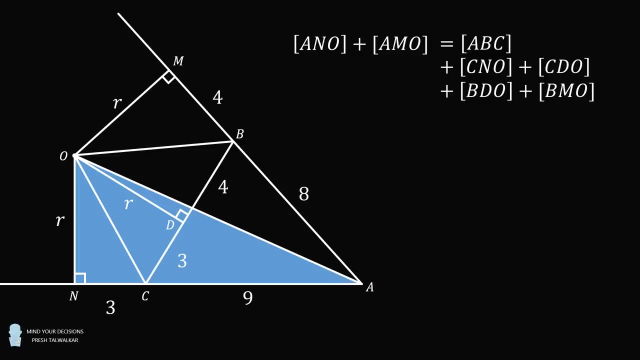 triangle BMO. So we add up all these areas, So we have two different ways of expressing the same area. therefore they're equal to each other. Let's now calculate each of these areas. The area of triangle ANO is equal to 12r over 2.. 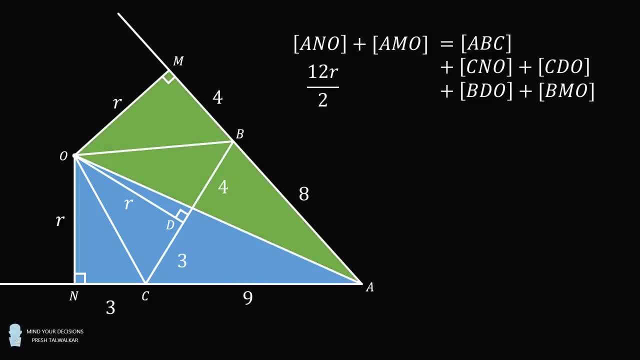 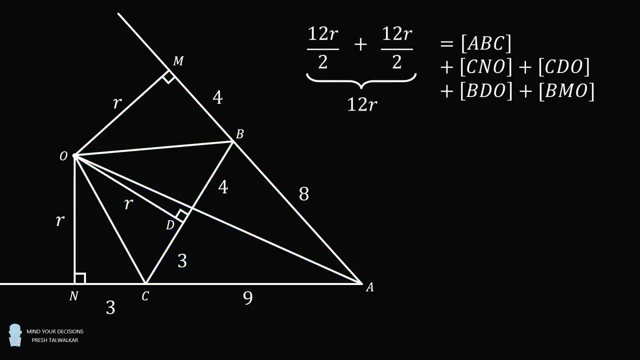 That will be the same area for the triangle AMO. We add these areas together and we get an area that's equal to 12r. Now let's calculate the areas of some of these other triangles. The area of triangle CNO is equal to 3r over 2.. 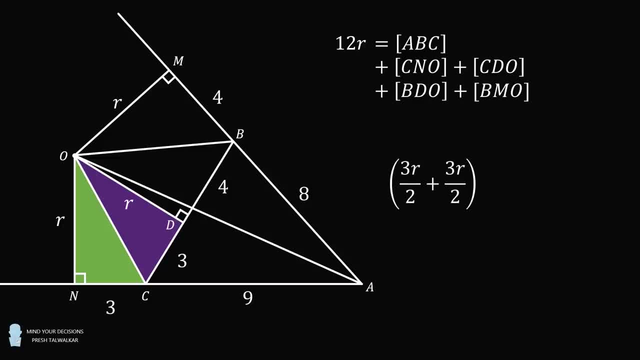 That's the same for the area of triangle CDO. We add these two areas together to get a total of 3r. Then the area of triangle BDO is the same of the area of triangle BMO, and each of these has an area equal to 4r over 2.. So in total their areas are equal to 4r. 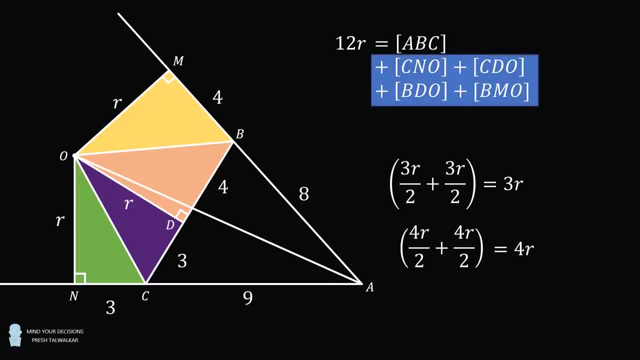 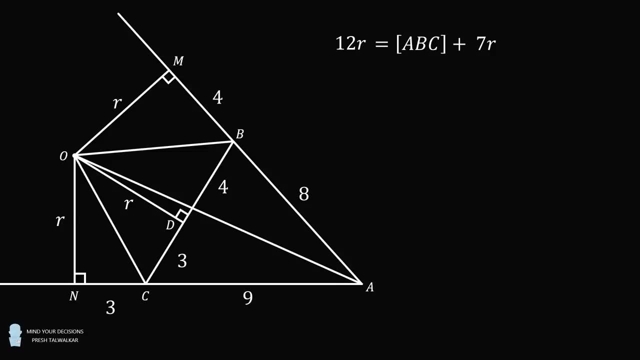 The total of all of these areas is equal to 7r. So we substitute that into the equation So we have 12r is equal to the area of triangle ABC plus 7r. So what's the area of triangle ABC? So what's the area of triangle ABC? 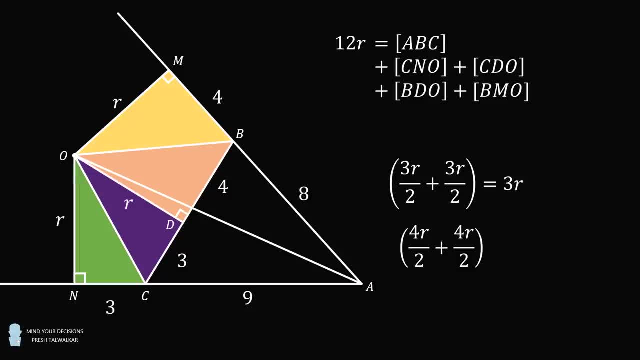 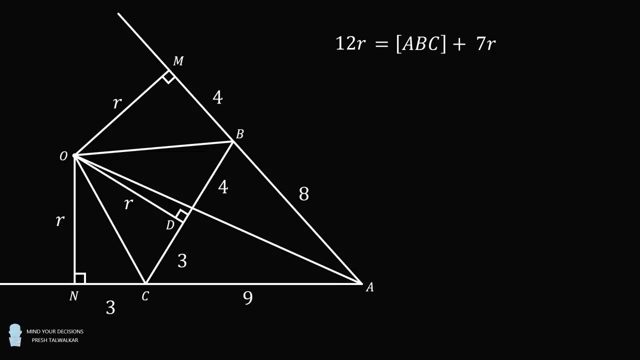 each of these has an area equal to 4r over 2.. So in total their areas are equal to 4r. The total of all of these areas is equal to 7r, So we substitute that into the equation We have. 12r is equal to the area of. 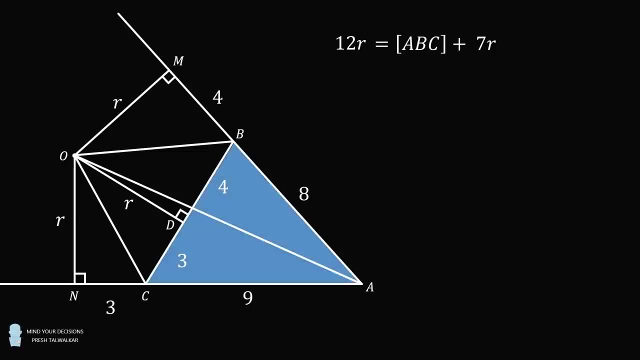 triangle ABC plus 7r. So what's the area of triangle ABC? ada thing is equal to 3 İstanbul ABC plus 7r Wilson. so what's the area of triangle ABC? We can solve for its area using Heron's formula. 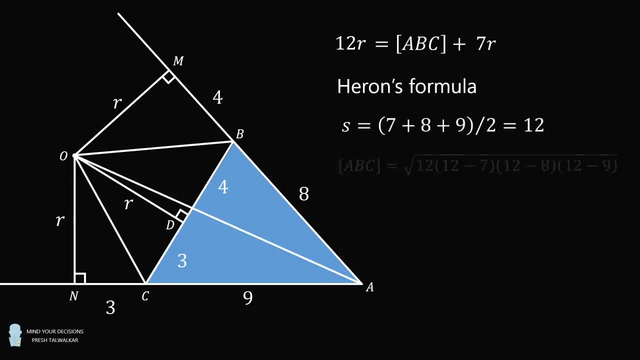 We first calculate the semi-perimeter and then we substitute into the formula. This is a straightforward calculation. We simplify under the radical to get the area of triangle. ABC is equal to 12 multiplied by the square root of 5.. So we substitute that into the equation. 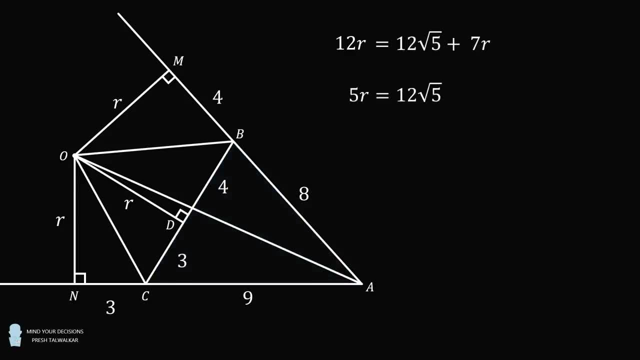 Then we subtract 7r from both sides to get 5r is equal to 12 times the square root of 5, which means r is equal to 12 times the square root of 5, all over 5, which is approximately equal to 5.367.. 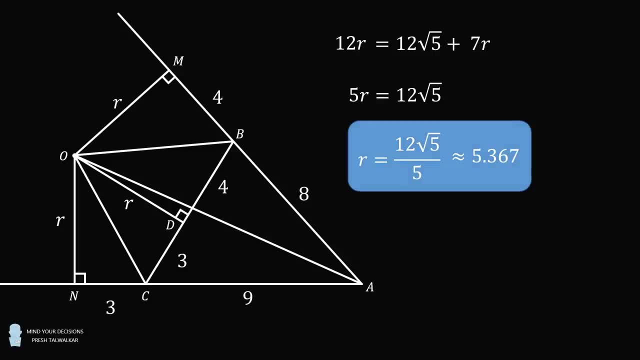 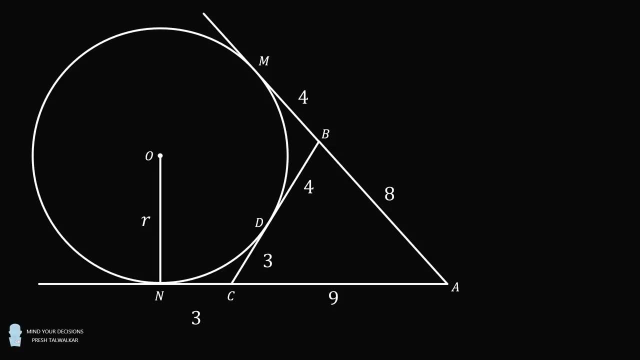 And that's one way to solve this problem. Let's now solve the problem using trigonometry. We'll start from this part of the derivation. We will again construct the following line: segment AO. This will divide angle A into two equal angles equal to 2.. 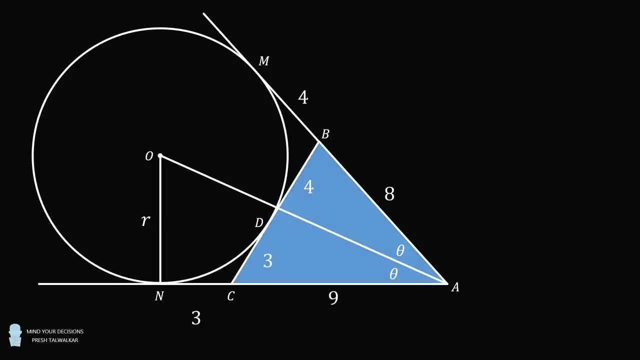 We'll use the angle 2 theta. From here we will consider triangle ABC to solve for the angle 2 theta. To do that we will use Alkashi's law of cosines. We have: BC squared is equal to AB squared plus AC squared minus 2 multiplied by AB, multiplied by AC. 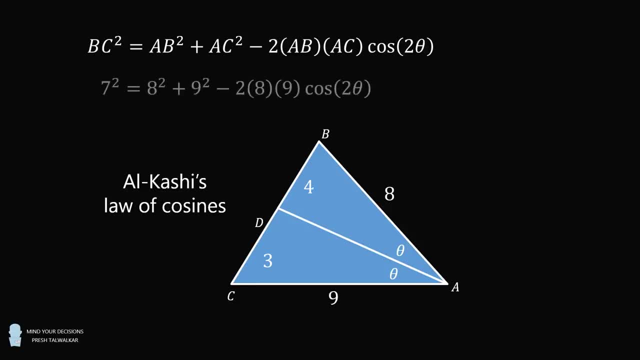 times the cosine of 2 theta. We substitute in the values and then solve for the cosine of 2 theta. This will be equal to 2 over 3.. We'll put that to the side for a second, and now let's consider the right triangle: ANO. 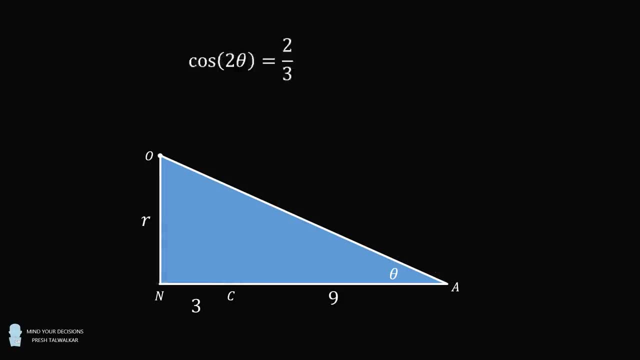 In this right triangle we have that r is equal to AN multiplied by the tangent of theta. We don't know the tangent of theta, so we'll use the tangent half angle formula and we'll use the form that involves the cosine of 2 theta. 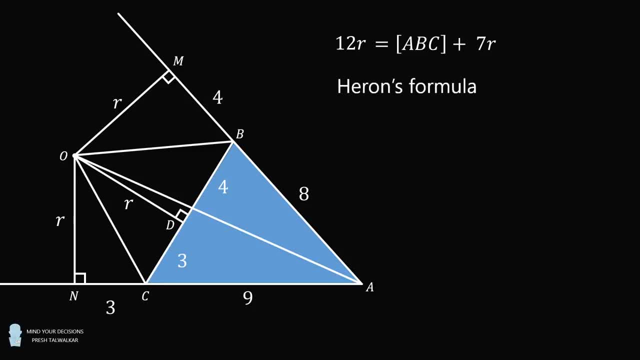 So what's the area of triangle ABC? We can solve for its area using Heron's formula. We first calculate the semi-perimeter and then we substitute into the formula. This is a straightforward calculation. We simplify under the radical to get: the area of triangle ABC is equal to 12 multiplied by the square root of 5.. 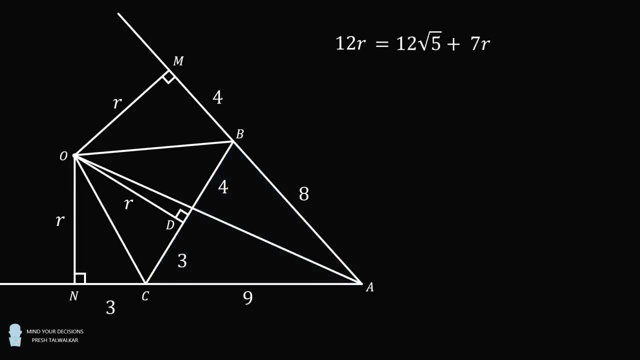 So we substitute that into the equation. Then we subtract 7r from both sides to get 5r is equal to 12 times the square root of 5, which means r is equal to 12 times the square root of 5, all over 5, which is approximately equal to 5.367.. 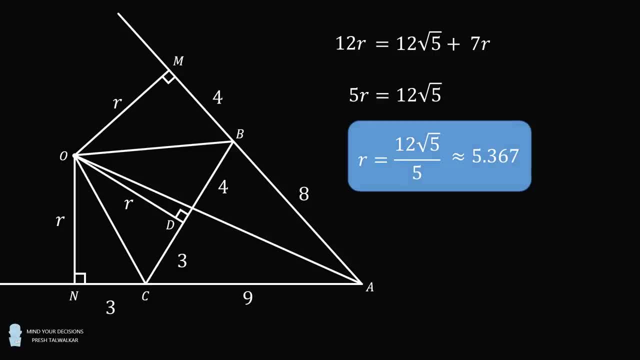 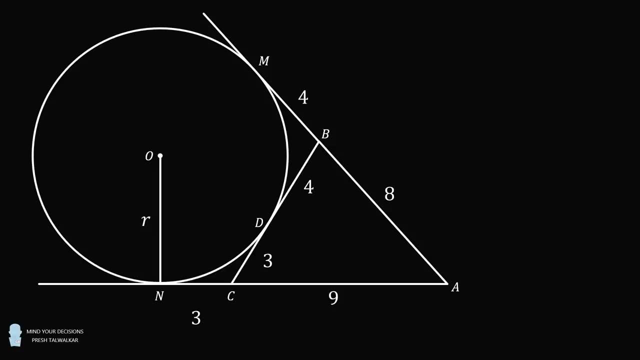 And that's one way to solve this problem. Let's now solve the problem using trigonometry. We'll start from this part of the derivation. We will again construct the following line: segment AO. This will divide angle A into two equal angles equal to theta. 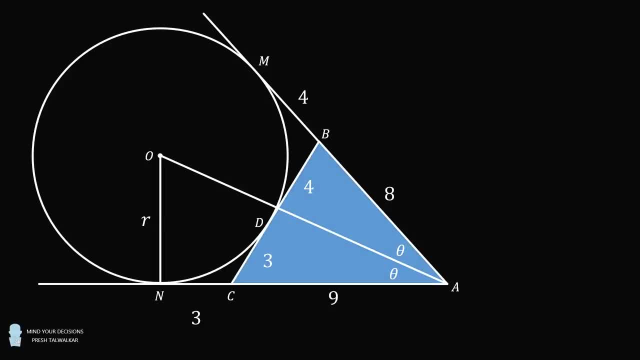 From here we will consider triangle ABC to solve for the angle 2 theta. To do that we will use Alcashi's law of cosines. We have: BC squared is equal to AB squared plus AC squared minus 2 multiplied by AB. 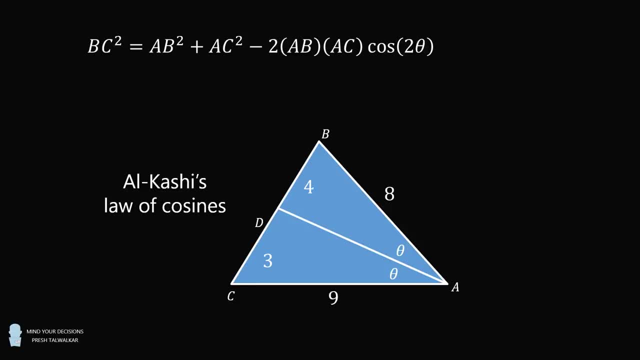 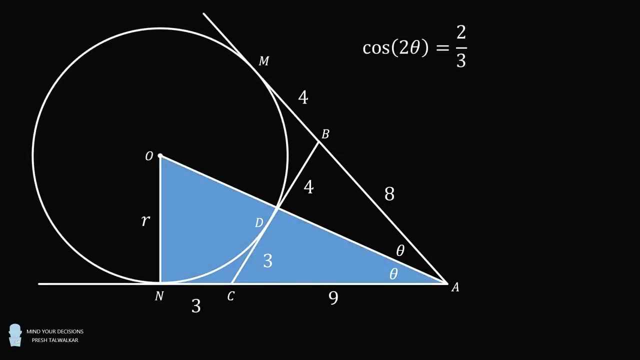 multiplied by AC times the cosine of 2 theta. We substitute in the values and then solve for the cosine of 2 theta, This will be equal to 2 over 3.. We'll put that to the side for a second, And now let's consider the right triangle: ANO. 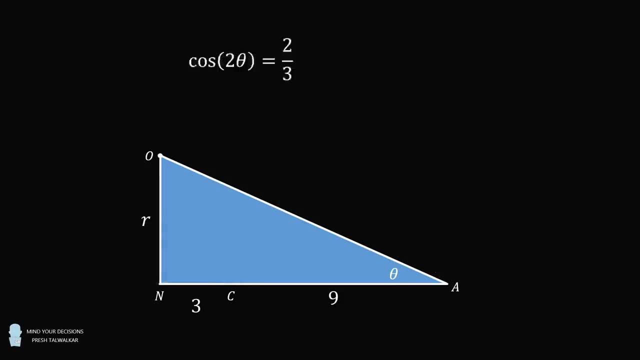 In this right triangle we have that r is equal to AN multiplied by the tangent of theta. We don't know the tangent of theta, so we'll use the tangent of theta, We'll use the tangent half angle formula and we'll use the form that involves the cosine of 2 theta. 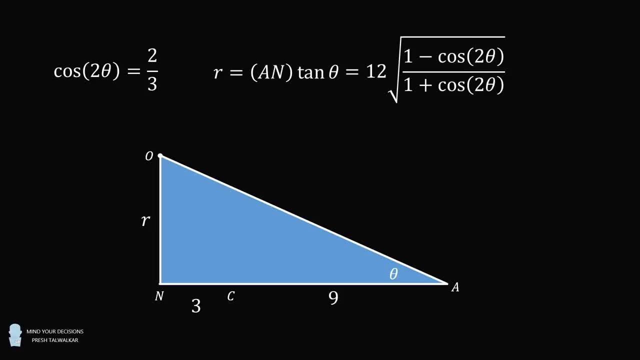 We also know that the tangent here will be positive because we have a positive radius. so we just take the positive square root. So AN is equal to 12 and we've substituted in the tangent half angle formula. We know that the cosine of 2 theta is equal to 2 over 3,. 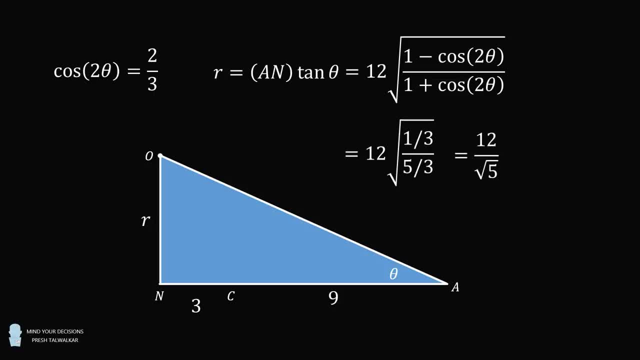 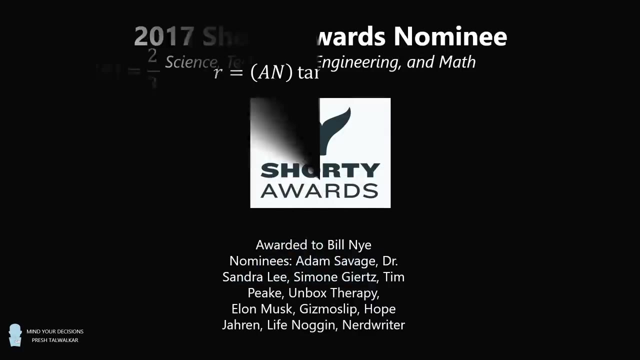 so we then simplify and this gives that r is equal to 12 divided by the square root of 5, which is is approximately equal to 5.367.. And that's another way to solve the problem. What an interesting question. Thanks for making us one of the best communities on YouTube. 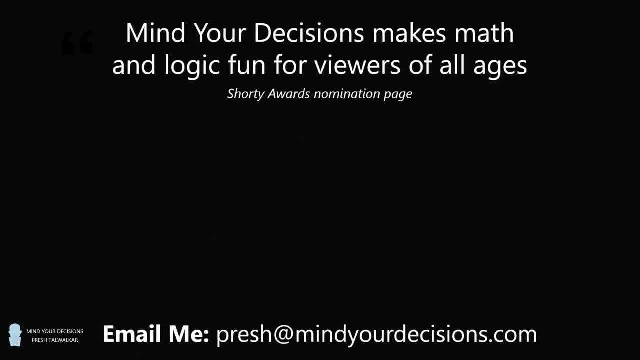 See you next. episode of Mind Your Decisions, where we solve the world's problems, one video at a time. you. 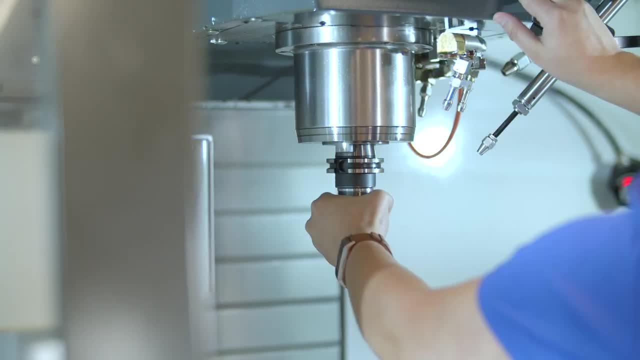 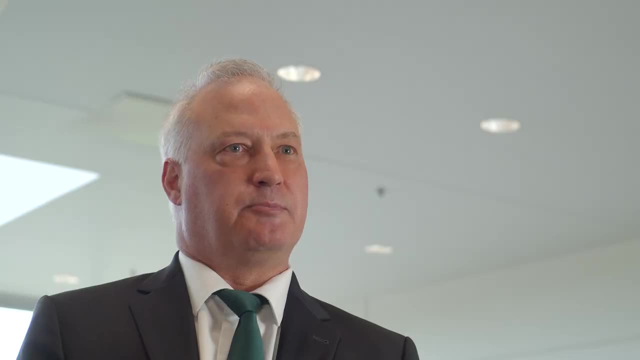 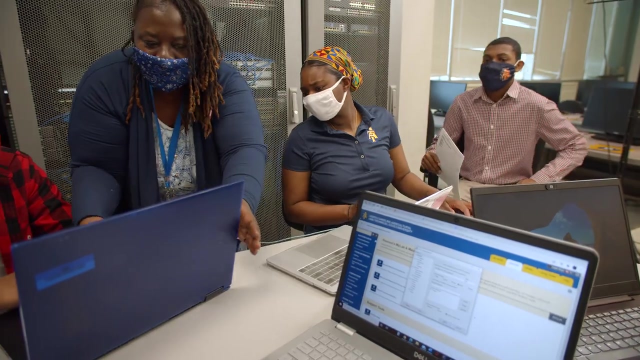 Welcome to the world of engineering technology. It's about solving real problems for real people, taking the best of the arts, the sciences, the humanities, blending them together into solutions, products that real people can use on a daily basis. Engineering technology students come to. 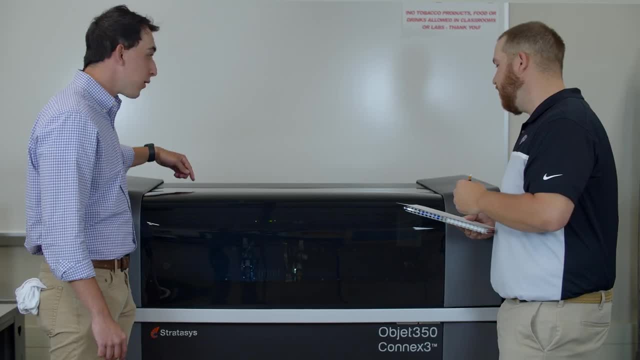 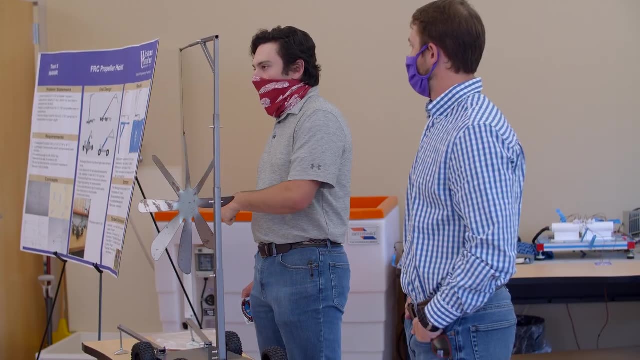 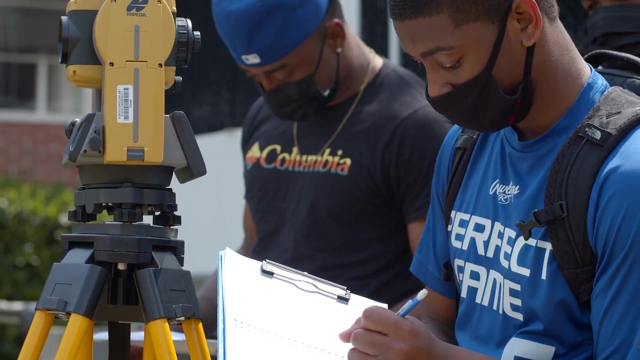 our programs with the desire to change the world. They want to make something special. so they come to apply their practical knowledge to hands-on problems. to get things done, To start the programs you don't need anything particular, but it really helps if you have a desire to learn and you've got interest in science and math. So there's often 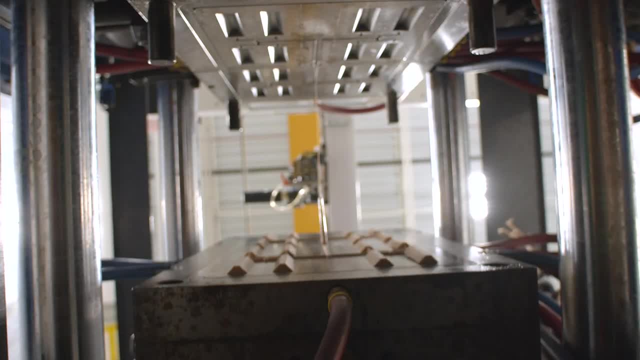 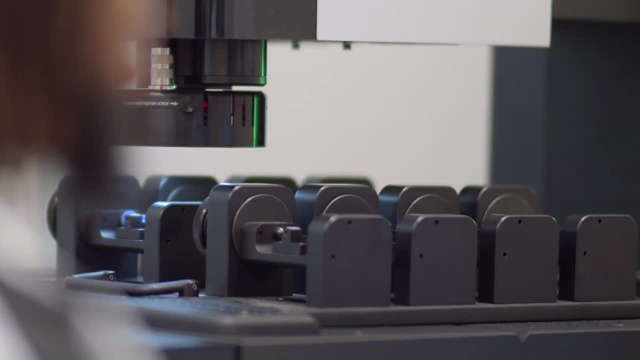 questions about the differences between engineering and engineering technology. They're both degrees that lead to careers in engineering, so engineering technology's the degree, engineering technology's the degree of engineering technology. The two of these are categories- engineering and engineering technology- but both degrees lead to careers in. 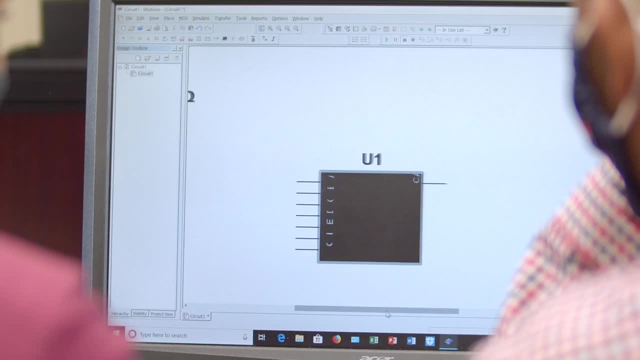 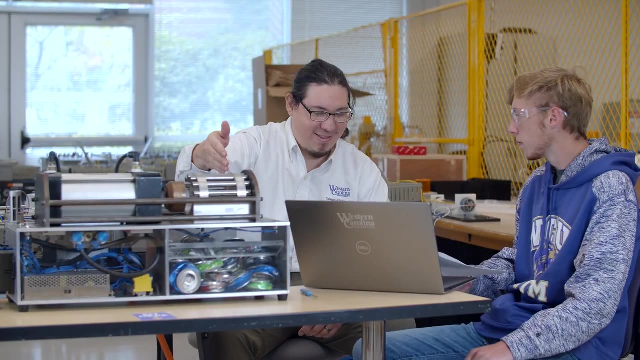 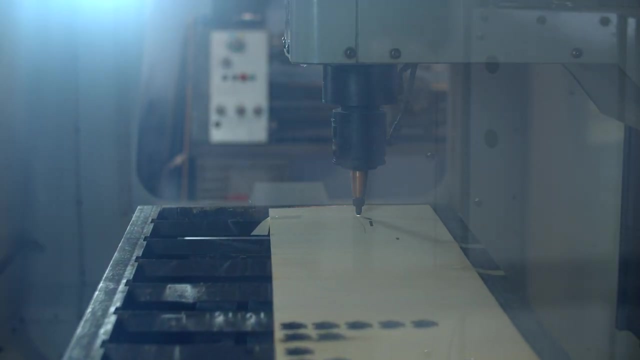 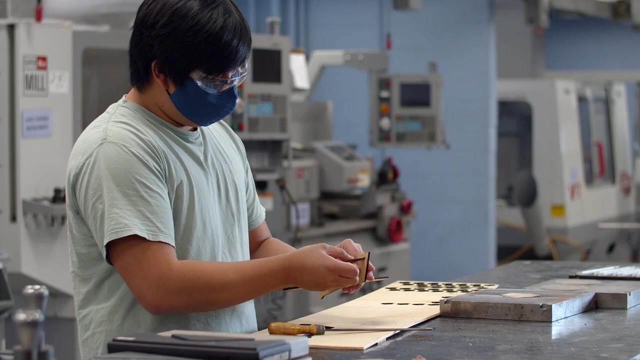 engineering is the career, So a majority of the states in the country have a pathway for engineering technology graduates to get a PE, a professional engineering license. Professional engineers come from all different backgrounds. The primary traditional path is engineering degrees, but engineering technology degrees are becoming increasingly common as a start for professional engineers. 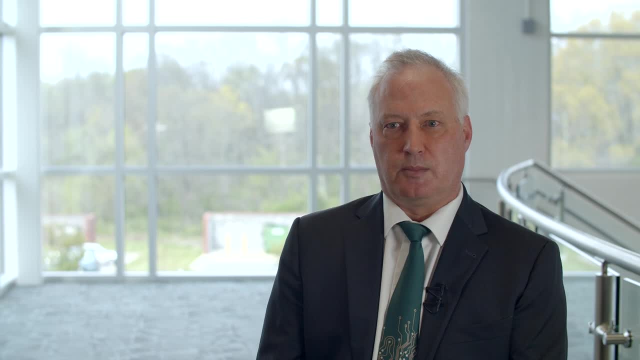 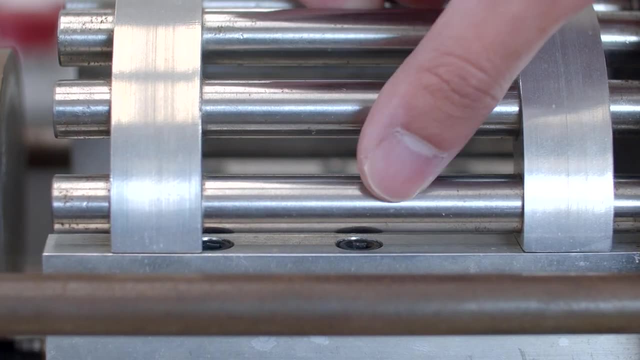 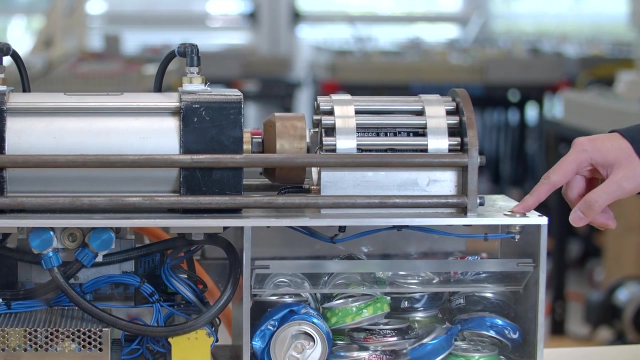 Engineering technology welcomes students from all areas to become part of the community, to make their mark on the profession. ET degrees quite often lead to management and other paths. With an ET degree you may start small but you can do huge things.